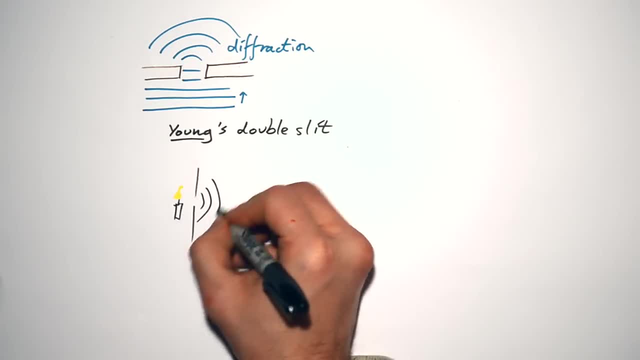 light went through the slit. Of course it diffracted like so, and then he had another two slits. These are Young's double slits right here. Why did he send the light through a single slit first? Well, he wanted monochromatic, coherent light to be coming out of these two slits here. 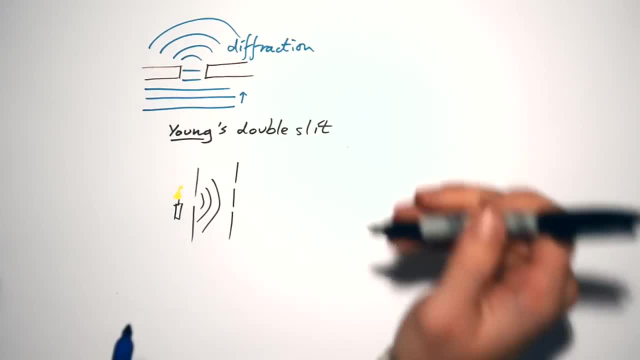 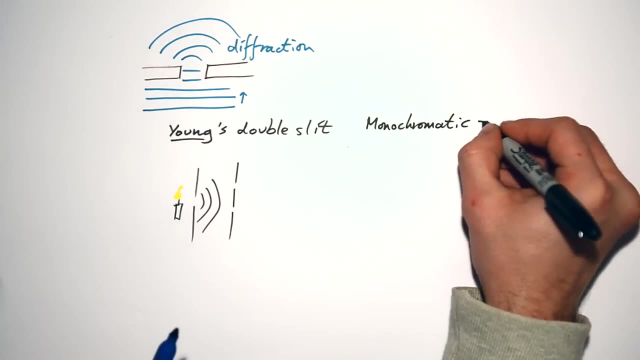 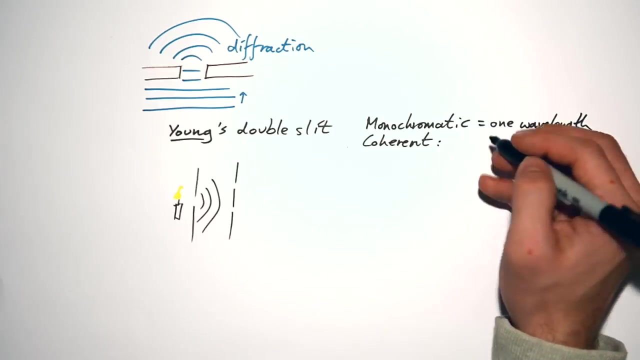 What does monochromatic mean? Mono, one chromatic colour, one colour or one wavelength. He wanted it to be coherent as well. Coherence also has this extra qualifier, which is constant phase difference. Now you might say that just means in phase. The light getting to these two points, these two slits, is in. 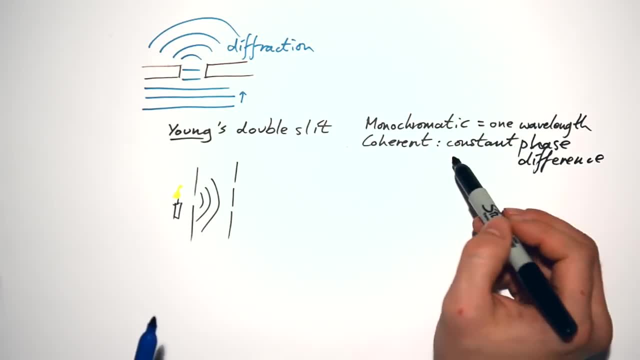 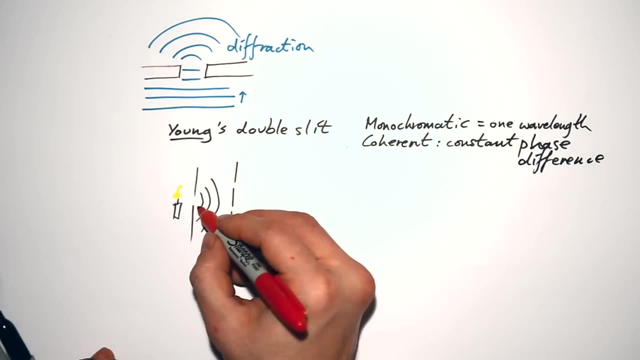 phase. but when the exams ask what does coherent mean? they like this monochromatic and constant phase difference definition, not just in phase. So what happens when light diffracts Longer wavelength light diffracts more Shorter wavelength light diffracts less. So in this case it would have been 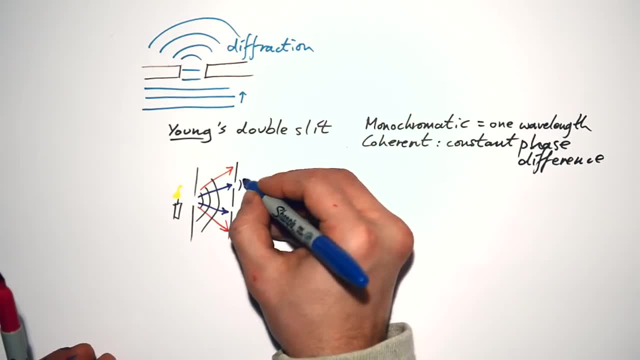 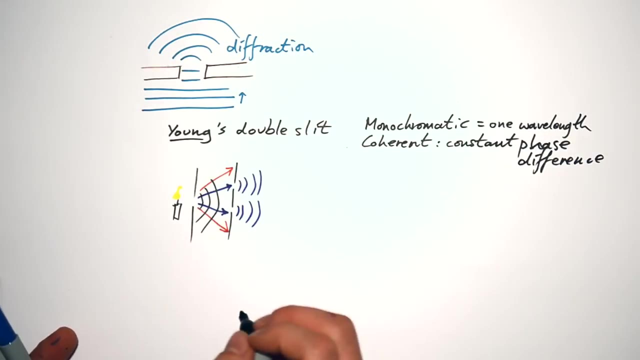 blue light that ended up coming from these two slits that Young had set up, Therefore making sure that there was only one wavelength coming out of there. Nowadays, we don't actually need this single slit, because we have lasers. Lasers produce monochromatic, coherent light, so we just bash that straight into our double slit. 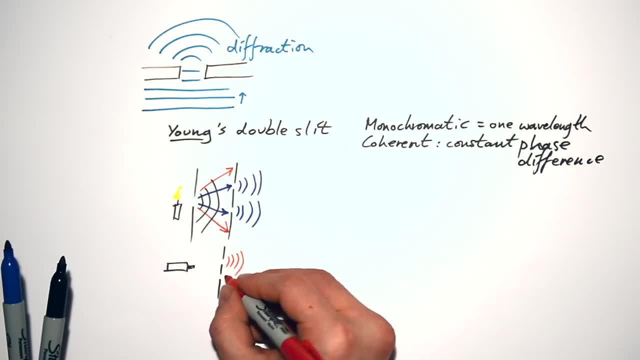 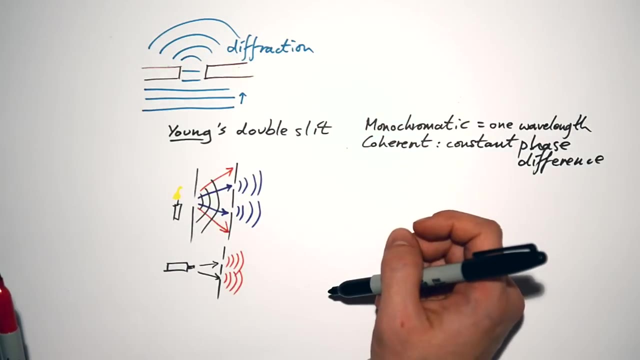 and we get the same effect. Generally we use red light, reddish light. So the difference between Young's setup and our setup nowadays is the only difference- is that he used a single slit to produce coherent light sources and we use a laser and a double slit. From then on, the whole experiment is exactly the same. Here we have our 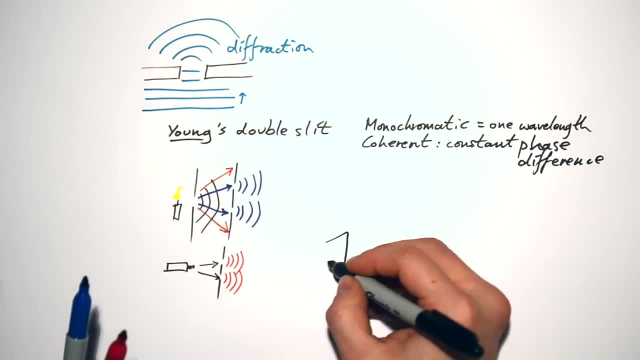 screen. Now, if I was to draw this screen in three dimensions, it would look something like this, like that: What do we see? Instead of just two spots being produced on this screen, in fact, we see a whole band of fringes made on our screen. Why is that? Well, that's because 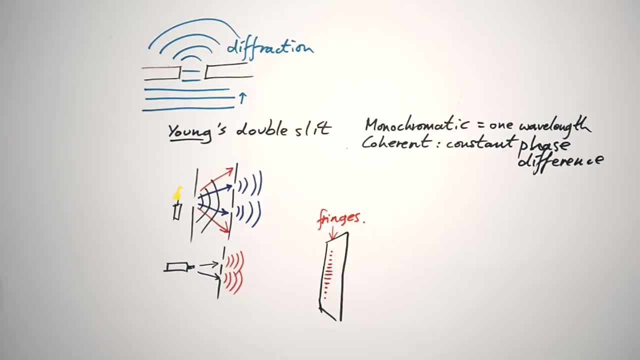 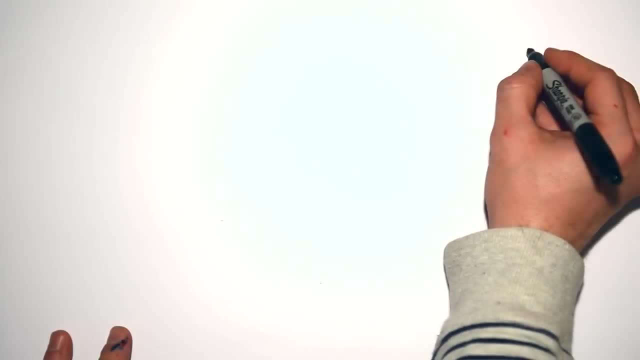 we have interference going on. We have super positioning. Let's make this a little bit bigger. Here's our screen, So here's our screen, So here's our screen. So here's our screen. Here's our screen here. and here's our double slits. 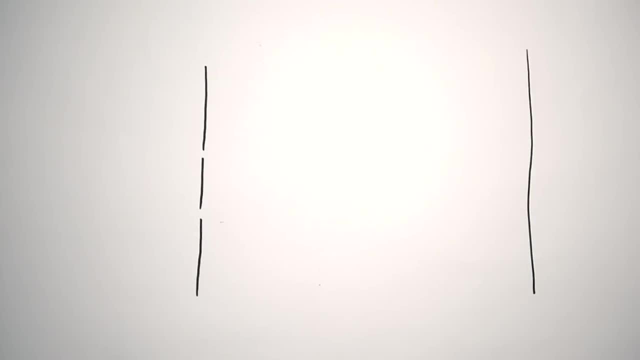 Now I'm going to draw light rays in different colours here, but that's just to show you the different light rays, but they should all be monochromatic in reality. So let's have a look at the waves that meet right at the centre. We have a wave coming from this top slit here. 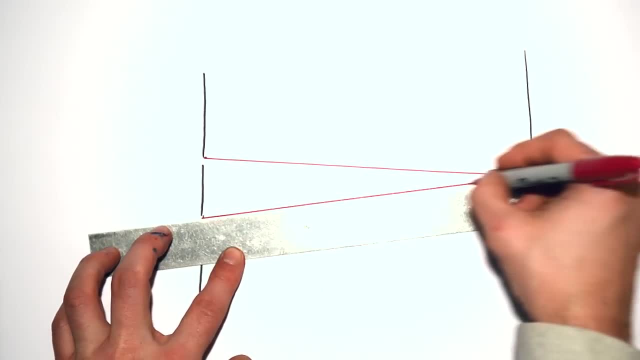 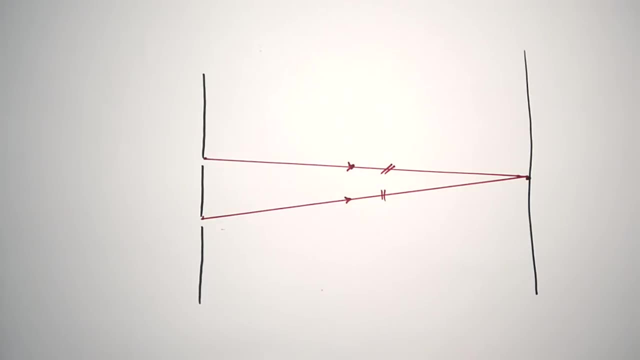 and we have a wave coming from the bottom slit here. Now these have travelled the same distance. We have just a normal isosceles triangle. So in other words, we can say the path difference is zero. That just means that they've travelled the same distance. Now, if they've travelled the 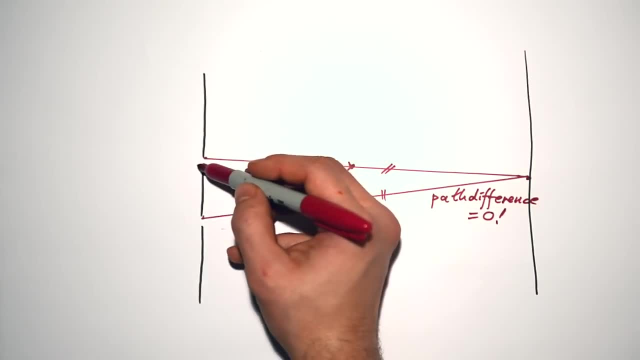 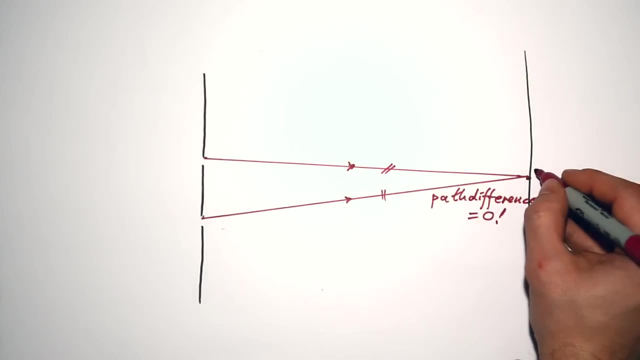 same distance. the waves arrived at the double slits in phase and they left the double slits in phase, So they'll be on the same distance. So that's a good sign- slits in phase. and if they travel the same distance at the same speed, then they've arrived. 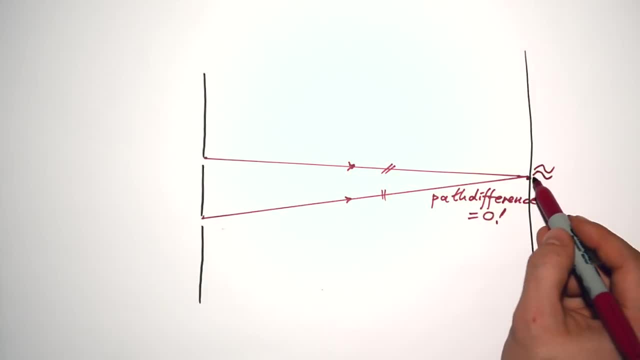 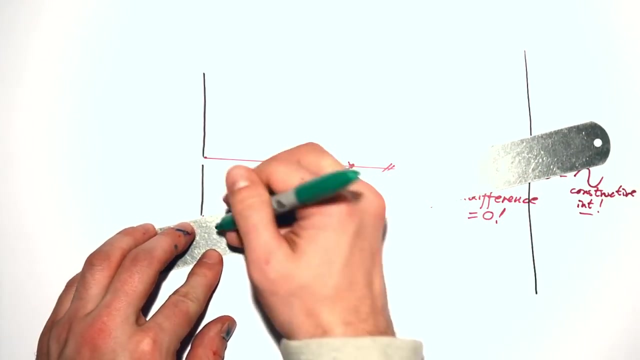 at the screen in phase as well. so i'm just drawing what they arrived at the screen. like if they superimpose, we get- we've just got- constructive interference. but they're not the only two waves leaving these two slits, are they? what about the waves that end up going to here? 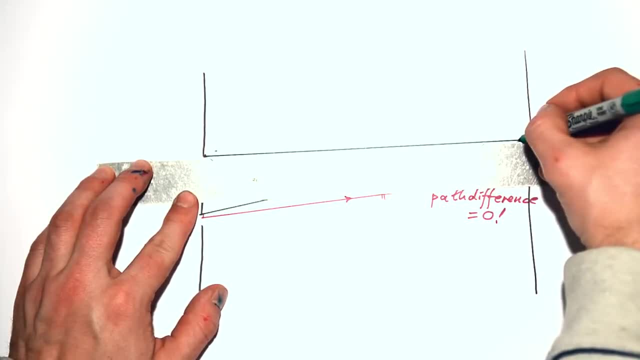 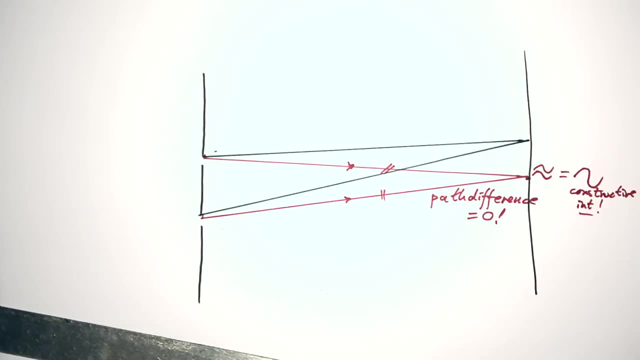 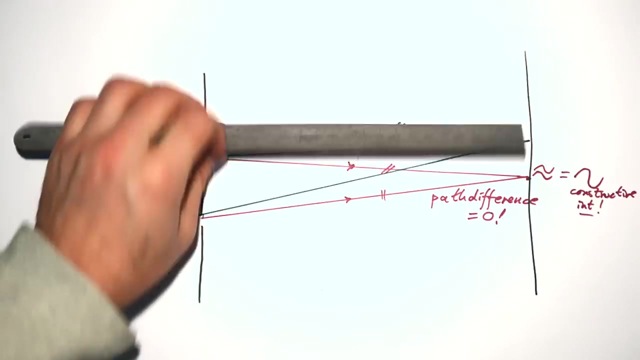 now, obviously, the ray coming from the bottom slit has traveled further than the ray coming from the top slit, so we do actually have a path difference this time. but what does that path difference equals to? well, if i take my ruler and i measure, that's 210. 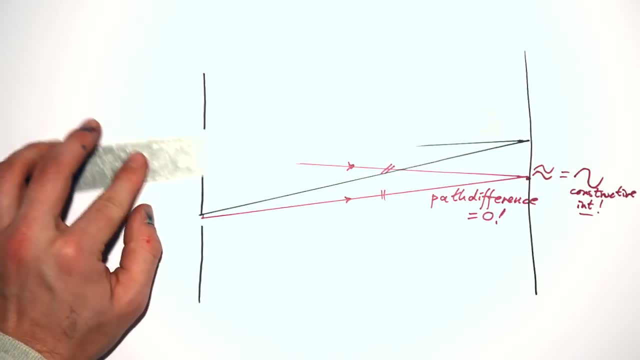 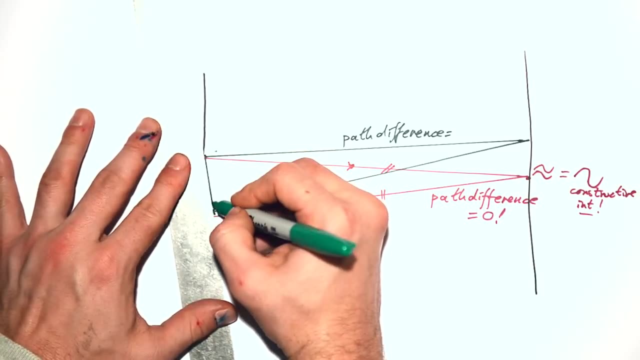 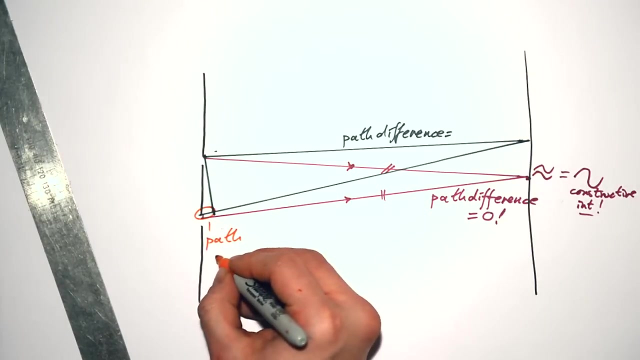 200, 10 on here. i can see that if i took this ray and put it onto this path here, it only comes to here. so if i draw a line there, this bit here is my path difference. that's how much further this ray has traveled compared to this ray. all i've done is make the right angle triangle there. 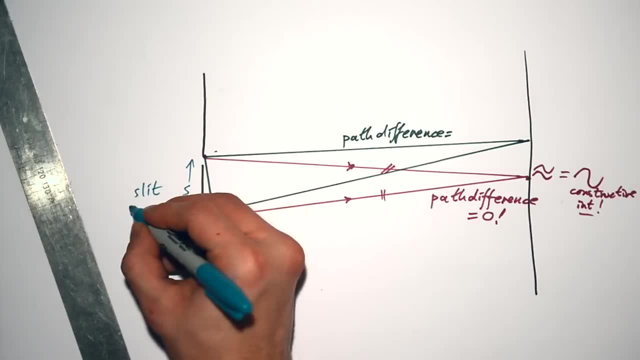 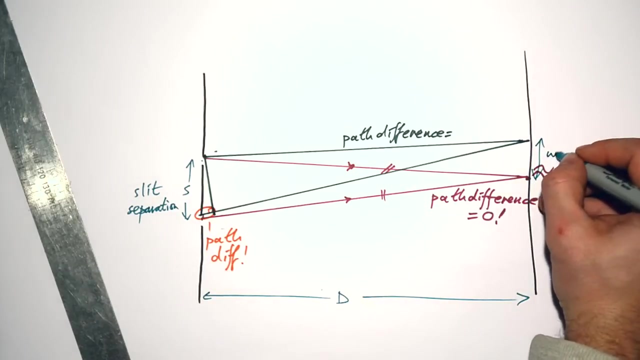 if we call this s, so that's the distance between the center of both of the slits. so from here to here, and i know that this distance here is- i'm going to call that- big d, so capital d, that's the distance from the slits to the screen, and i have my width here between one bright fringe, that's in the center. 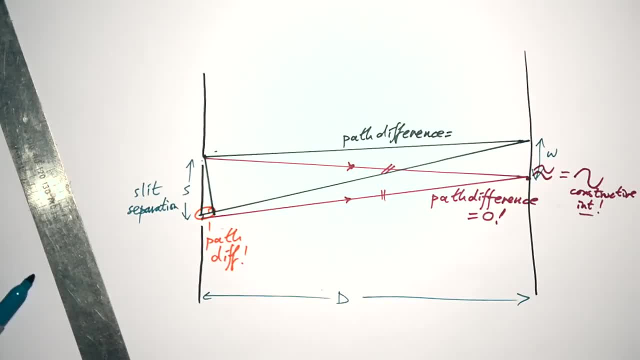 because we have constructive interference there, and my next thing we're going to do is i'm going to bright fringe, which also must mean that these waves are arriving in phase and constructively interfering as well- Then, using some clever trigonometry- you don't really need to know the derivation for this- 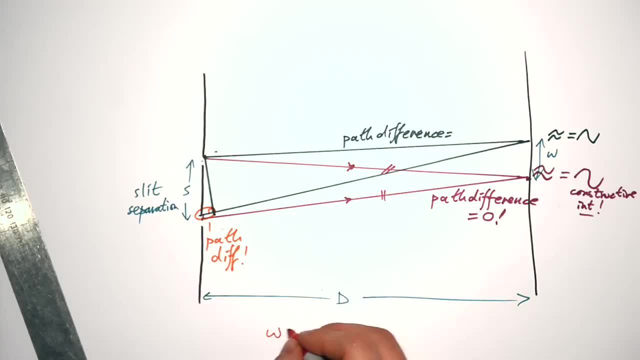 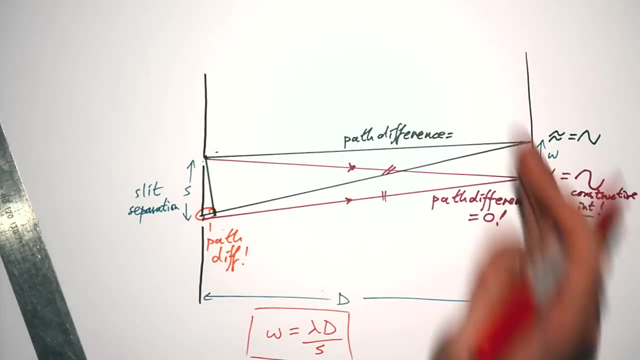 we come up with Young's double slit equation, That is, W equals lambda D over S. This is a slight approximation, so it doesn't work perfectly. it gets less and less accurate the further away from the screen you get, because it assumes that we have a curved screen when in fact we actually don't. we have a flat. 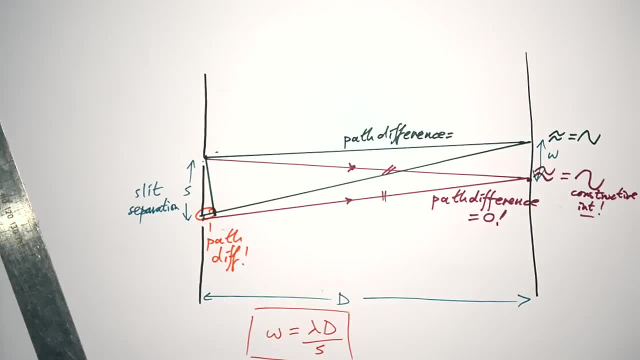 screen Now. the only way that this can be true is if the path difference here is exactly the same as the wavelength of the light. So if this ray has travelled one wavelength further than this ray, that means that it's still going to arrive in phase. 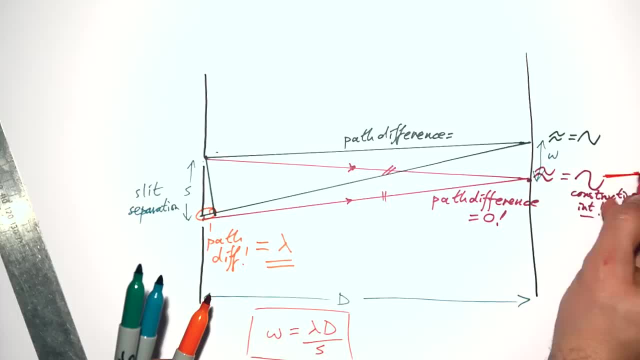 So that's why we get a bright fringe there as well. So we've got a bright fringe here, I have a bright fringe here. What's going on in between? when we have a dark fringe, Does that mean there's no light hitting that point on the screen? 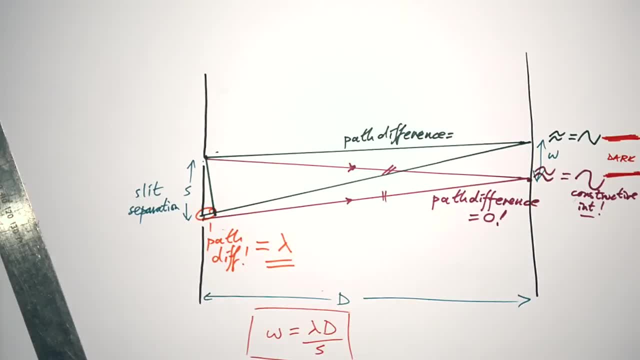 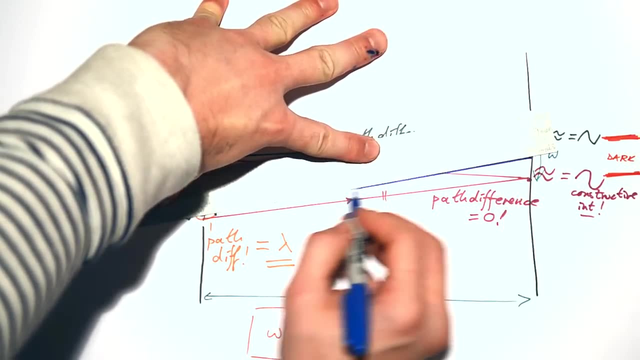 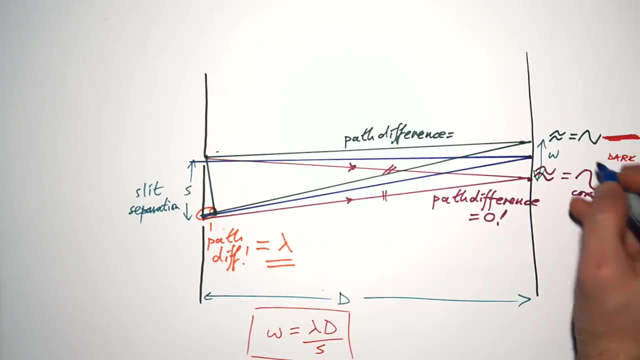 Of course not, because there's light hitting all points on the screen here. So what is happening in reality is that we have this ray and this ray, and this time the path difference is by length. Okay, That's wet, Nothing really. 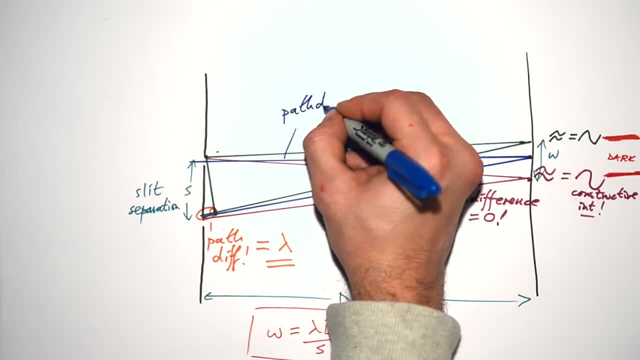 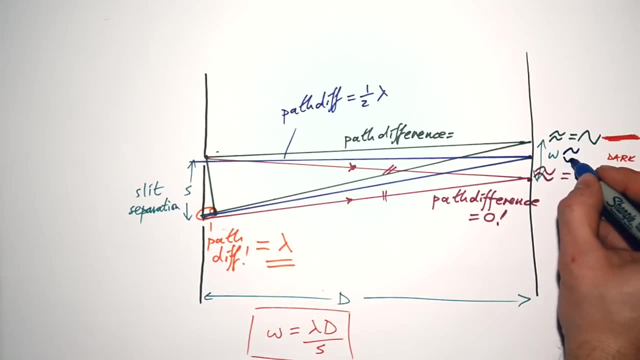 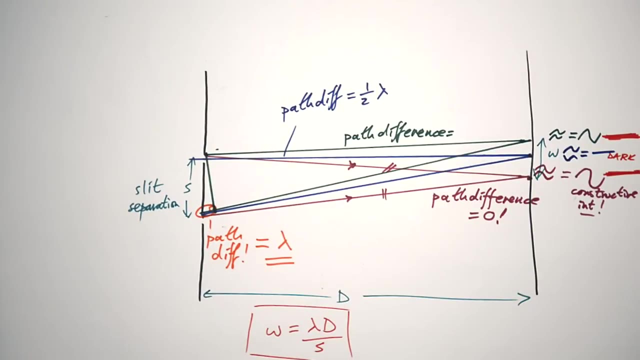 Everything is dark, Everything is wet is half a wavelength. What does that mean? It means that the waves actually arrive pi radians or 180 degrees out of phase. They don't constructively interfere, they destructively interfere, They cancel each other out and we end up with a dark spot. So light is reaching. 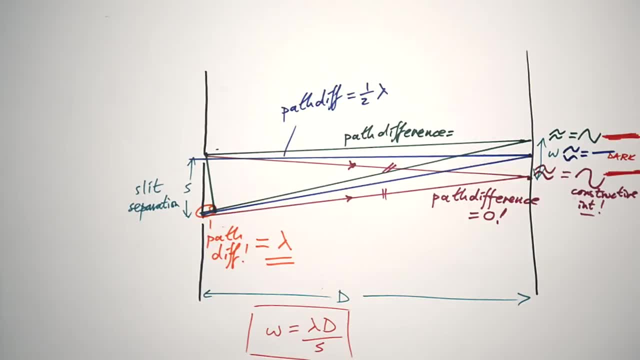 that point on the screen, but when the waves superimpose, no light is reflected off the screen. Quite trippy, but that's what happens. So if the path difference is a multiple of the wavelength, one lambda, two lambda, three lambda, four lambda. In other words, if one 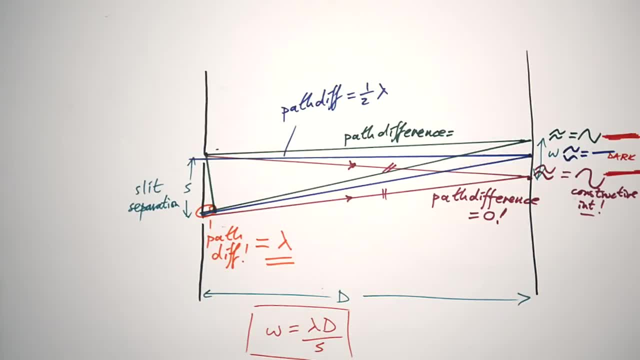 of the rays travels a multiple of the wavelength further to get to the point on the screen than the other ray, then you end up with constructive interference because the rays arrive in phase. If the path difference, however, is a multiple and a half of the wavelength, then that means 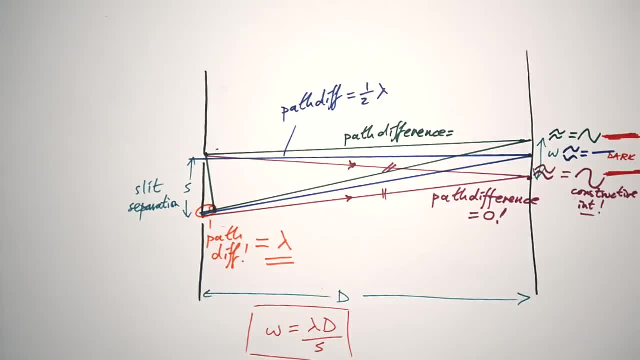 that the waves are going to arrive out of phase. pi radians 180 degrees out of phase. So that means that you end up with constructive, That means that you end up with destructive interference. So that's, when you get a dark fringe Constructive interference, you end up. 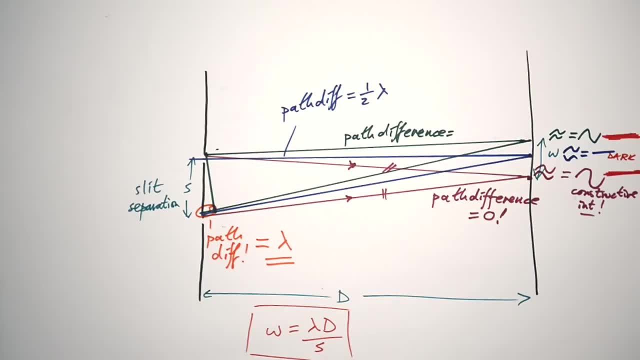 with a bright fringe. Dark fringes are because of destructive interference. When you're measuring these experimentally, it's very difficult just to measure one fringe. So what you do is measure at least 10 fringes using the dark fringes, because they're much easier to see, and then 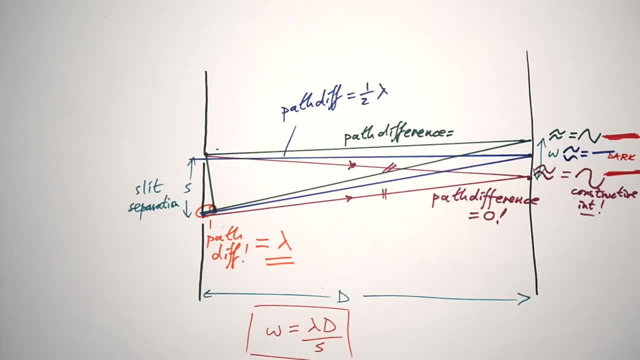 divide by 10 to find the mean fringe width. It's worth making sure that you understand how all of these things relate to each other, As W is inversely proportional to S. if lambda and D stay the same, that means that if S doubles, W halves, and vice versa as well. 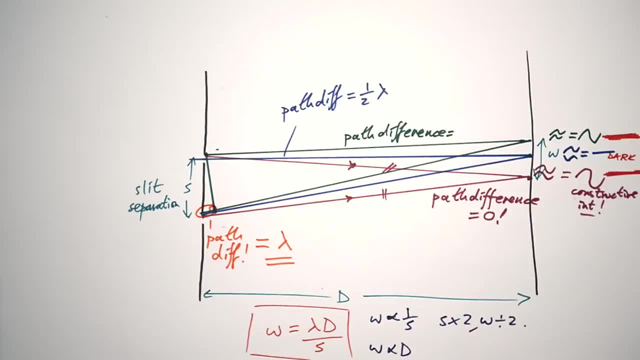 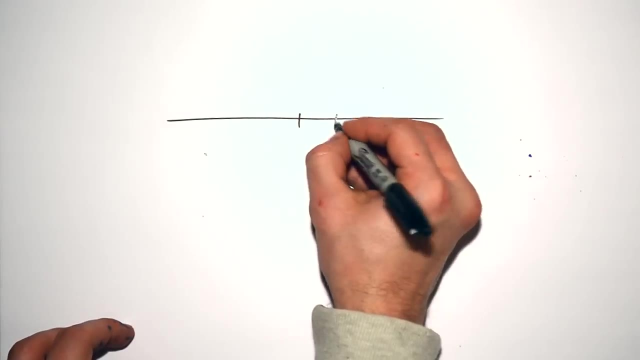 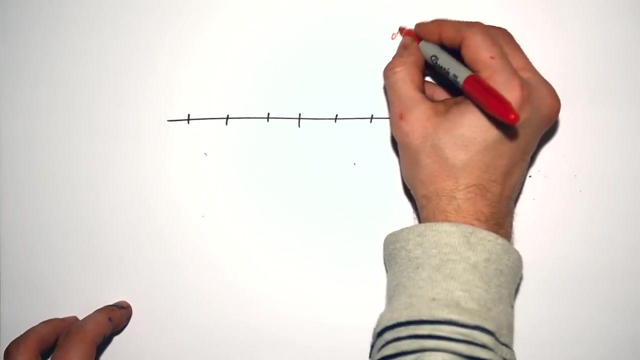 Also we have W is proportional to D if lambda and S stay the same. So that means that if D doubles, the fringe width has to double as well. One aside regarding this: If we draw what the interference pattern looks like for the double slit, 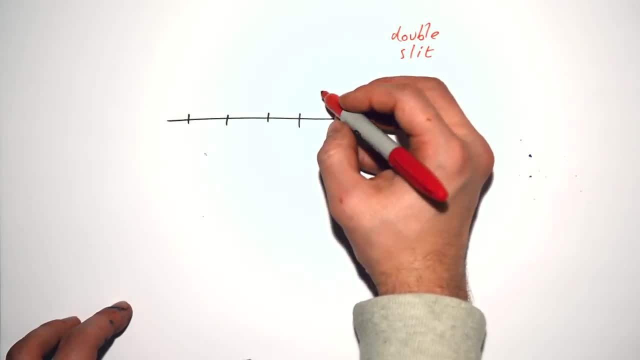 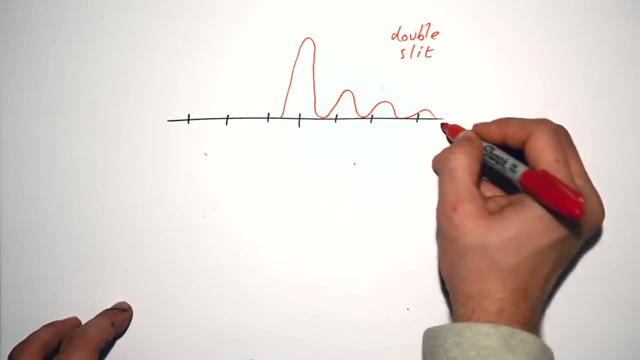 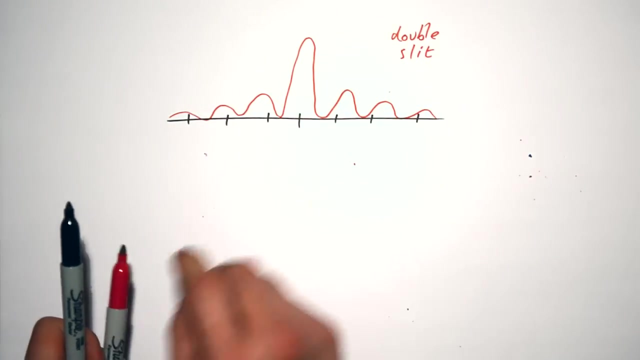 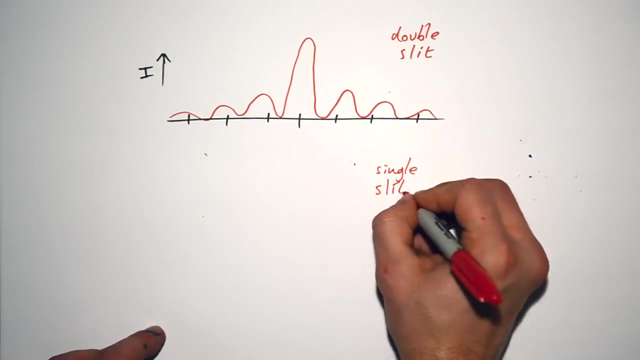 we see this happening: Each fringe width is the same size and the intensity of the fringes drops off fairly slowly. However, we do actually get interference from diffraction from a single slit as well. All you need to know is that if you're measuring a single slit, you need to know that if you're 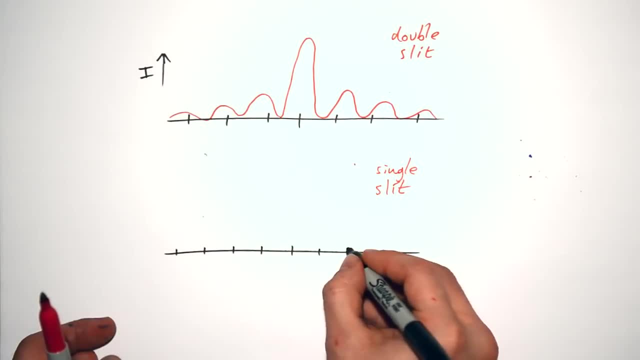 measuring a single slit. you're measuring a single slit. The difference between the two is that the interference pattern changes. thusly, In this case, with the single slit, central max is a central bright fringe. the central maximum, Central maximum, is very intense, very bright. 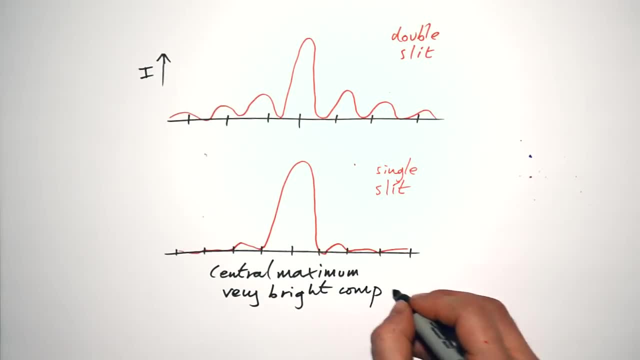 You can see that this is a synchronised interface of the two fringes compared to the other fringes, And also it is double the width of the fringes too. So that's all you need to know about. the single slit is how the interference pattern differs from. 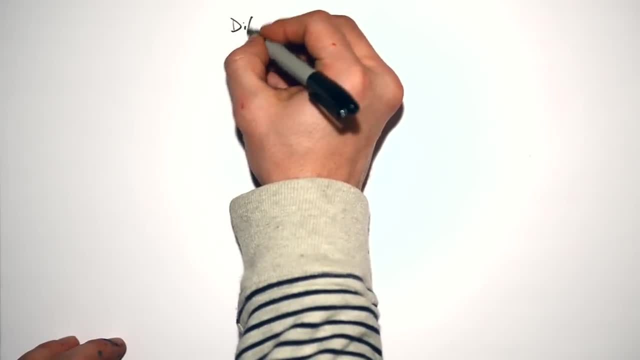 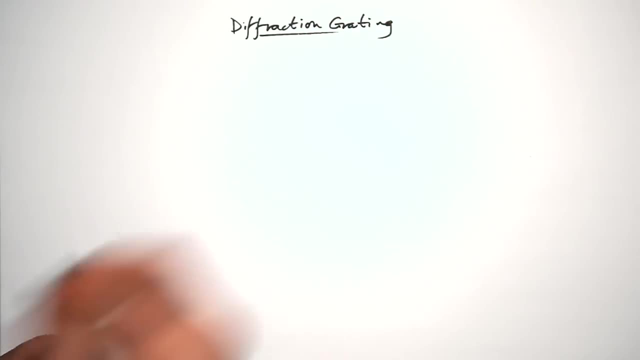 the double slit. So how is a diffraction grating different to each other? Well, the difference is very Young's double slit Instead of just having two slits like that. instead we've got loads and loads of slits that are very, very small and we get lots and lots of diffraction happening. 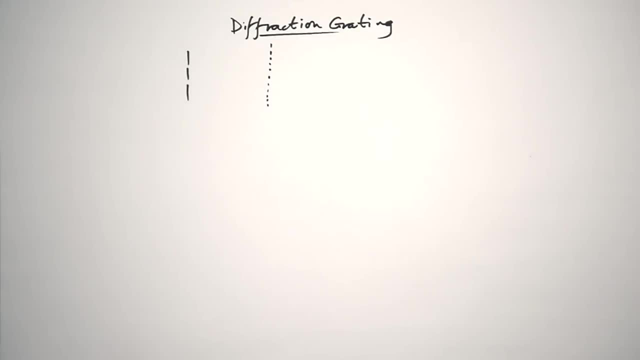 when light passes through that and diffracts afterwards diffracts as it goes through. This is where we can't use Young's double slit equation. we actually have to use a new equation, and now it's sort of interchangeable and it's a more accurate version of Young's. 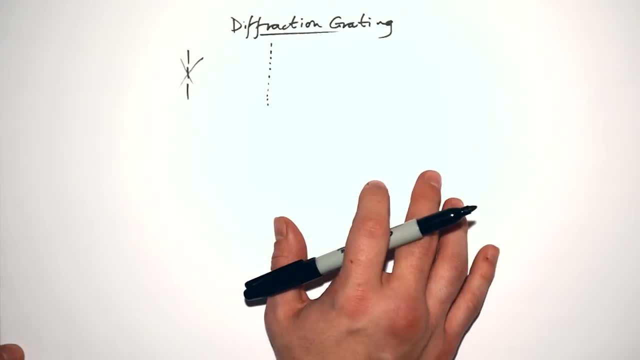 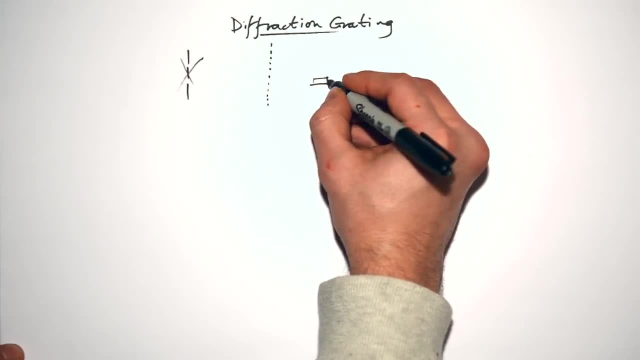 double slit equation, but we use Young's double slit equation for the double slit and we use this equation for the diffraction grating. So let's say we have our laser there and it's firing light towards the diffraction grating like so, and there's our screen. We actually 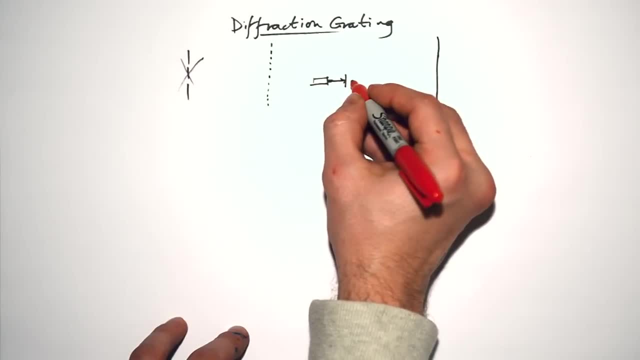 get so much diffraction in this case that we end up with very visible orders. So one, two, three, four, five, six, seven, eight, nine, ten, eleven, twelve, twelve, thirteen, nineteen, twenty, twenty-one, twenty-two, twenty-three, twenty-three, twenty-four, twenty-five, 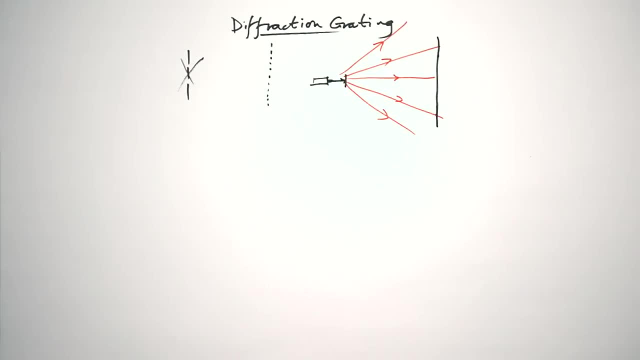 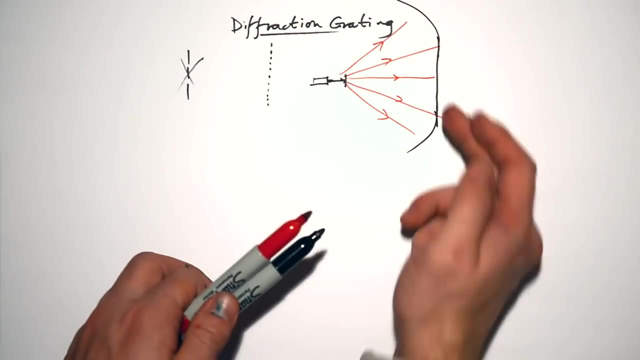 twenty-six, twenty-seven, twenty-seven, twenty-eight, twenty-nine, twenty-eight, twenty-nine, twenty-nine, twenty-eight, twenty-nine, twenty-nine. Might get a few more like that. Now, technically, I should draw this with a curved screen, because we are going to be dealing with angles instead. 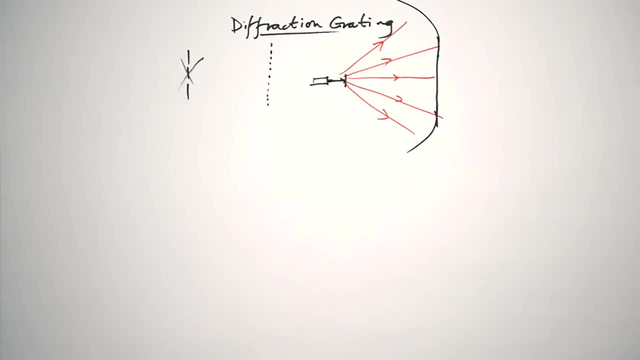 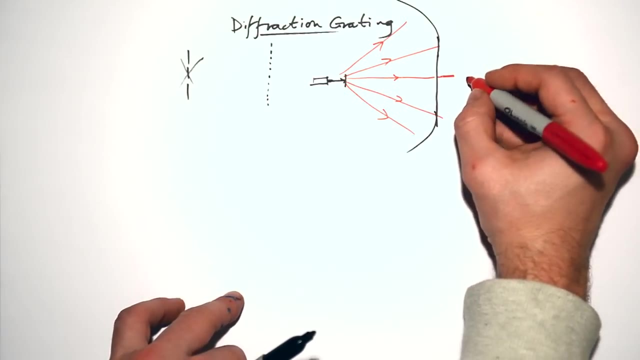 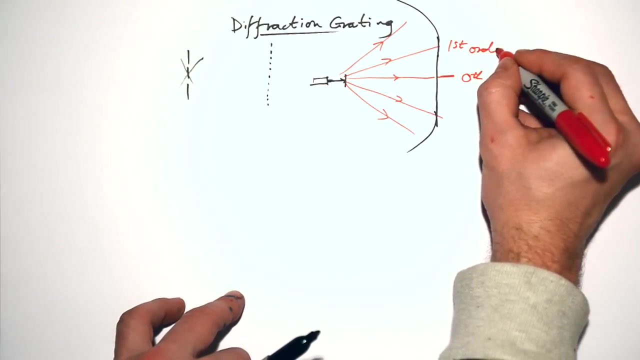 of fringe width in this case. that's why we can't use Young's double slit equation. The order, the bright fringe that we get on the screen at the centre, the central maximum, we call that the zeroth order Going outwards, we call them the first order, first order. 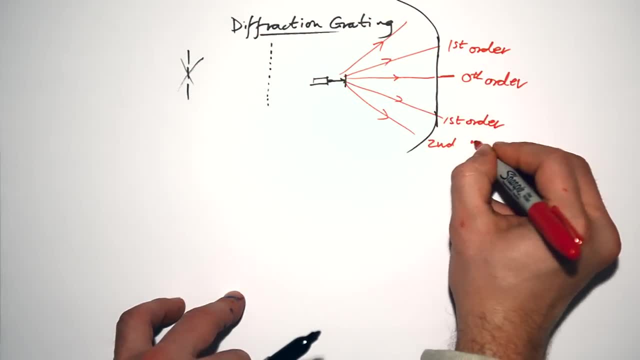 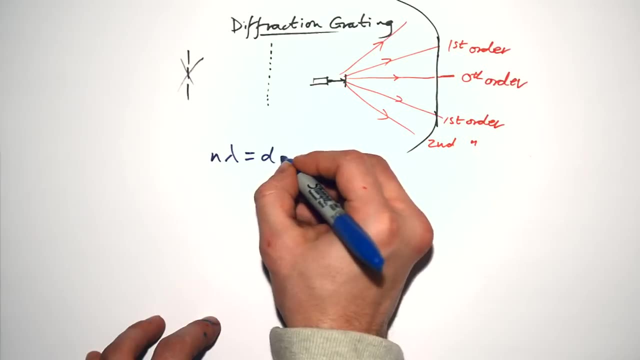 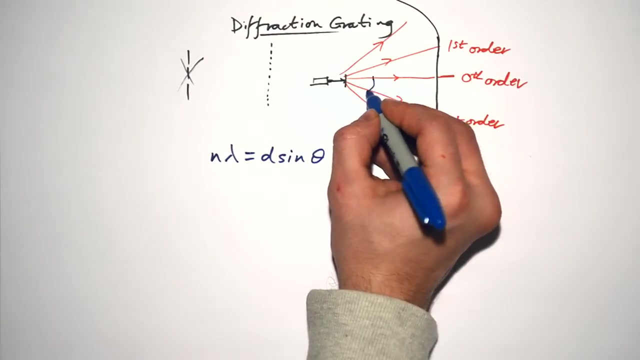 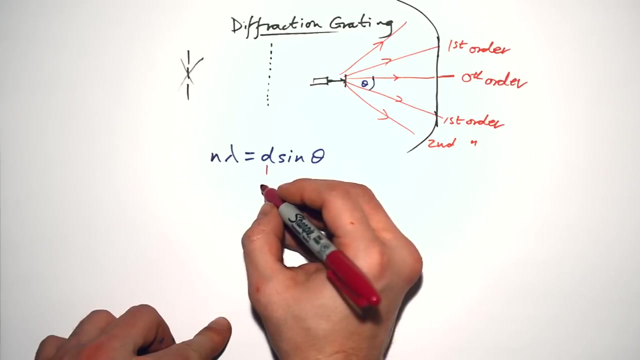 side as well. second order, and so on and so forth. the equation that we have is n lambda equals D sine theta, theta being the angle between the central zeroth order and that order. we might be looking at the first one, we might be looking at the second one or the third. so this is our angle, D is our slit width in our 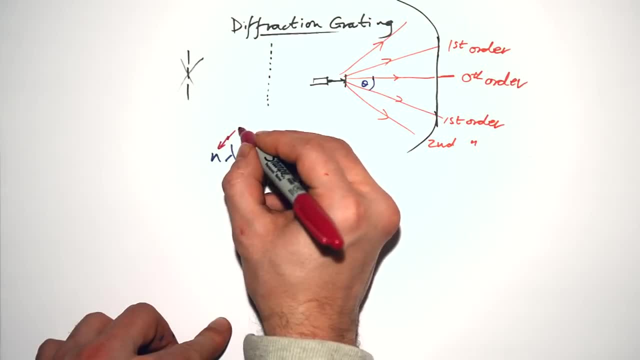 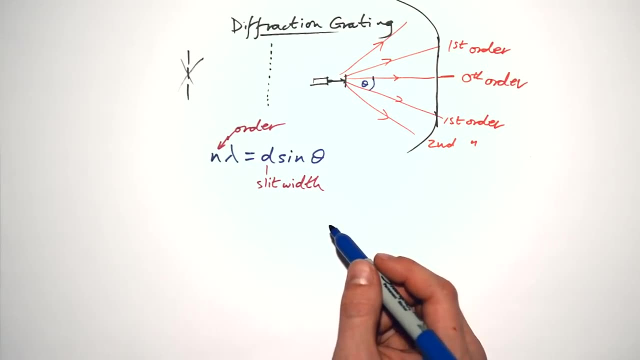 grating n is the order that we're looking at and obviously lambda is our wavelength. still now, one of the problems is is that the size of D in this case is so small that it's not really that helpful to write it on our diffraction grating. 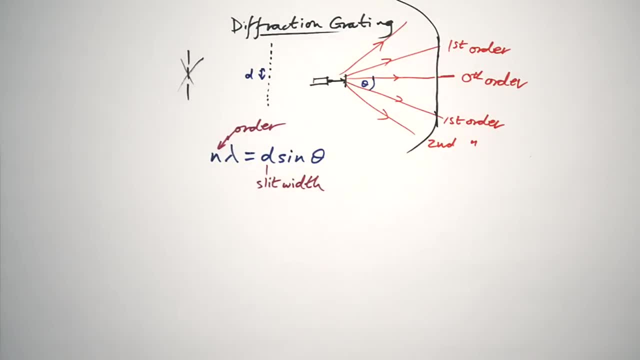 sometimes you'll be given big D instead. now this is where you have to be really, really careful, because big D is not the distance D for grating. it is lines per, usually per millimeter. so let's say that we have a, a grating that gives us 100 lines per millimeter. we don't want lines per. 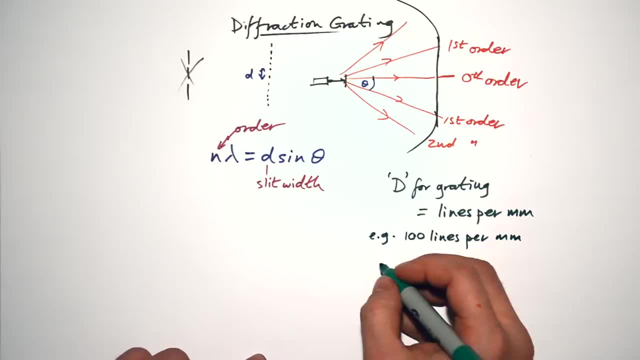 millimeter. we just want to know how big one of these lines is. what do we do to find little D? we just take the reciprocal. so it's going to give us one over a hundred, just going to give us not point naught, one millimeters, bear in. 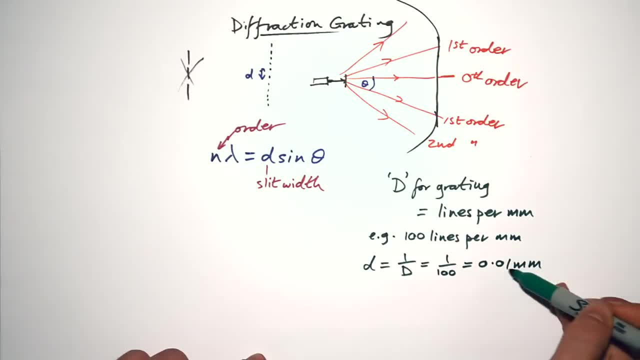 mind that whatever it says- lines per, whatever unit, that's how big the line is- the measurement is going to be for your slit width, your slit separation, for your grating as well. you obviously need to turn that into standard form, into meters. so it's going to be at the minute is 1 times 10 to the minus 2 millimeters. so 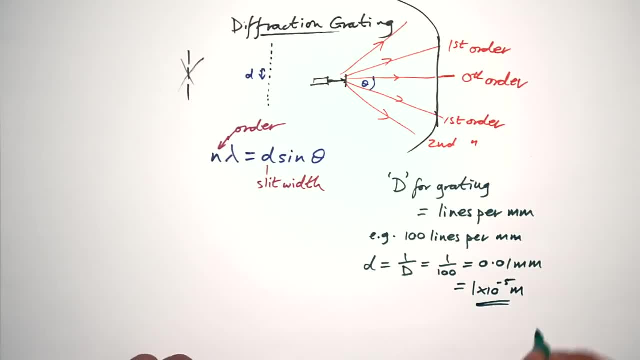 it's going to be 1 times 10 to the minus 5 meters, so you always, always need to turn it into meters in order to use it in the equation. here I can tell you the angle of the second order, so I'm going to put theta. 2 is actually 50 degrees. 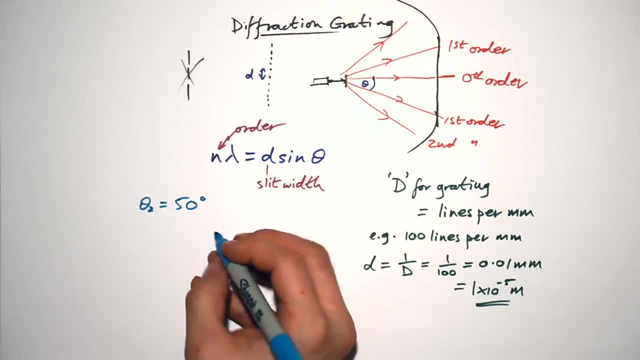 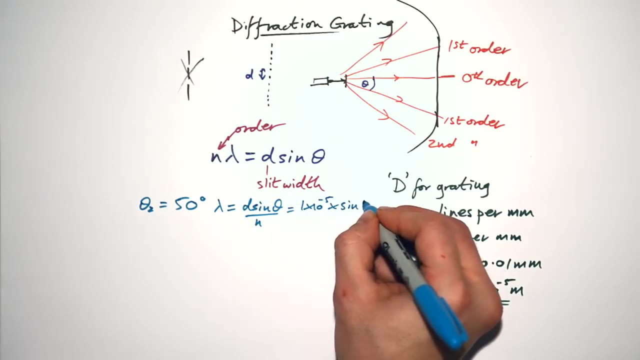 because that's my second order. if I'm trying to find out the wavelength here, I'm going to do: lambda equals D sine theta divided by n. that's going to be our separation there: 1 times 10 to the minus 5 times the sine of 50 degrees. 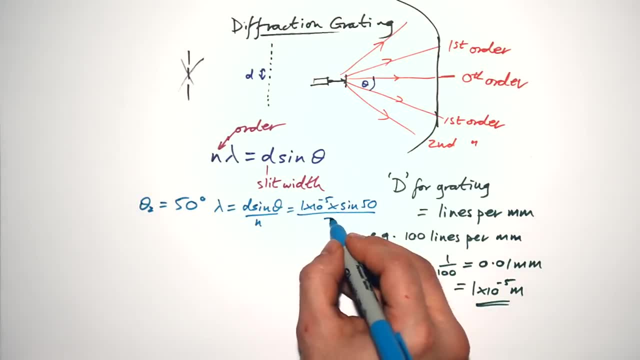 make sure you are in degrees, not radians, and then divide that by 2, because that's the angle of the second order. so I'm going to put theta: 2 is actually 50 because that is the second order. I'm looking at this: 50 degrees, right here. 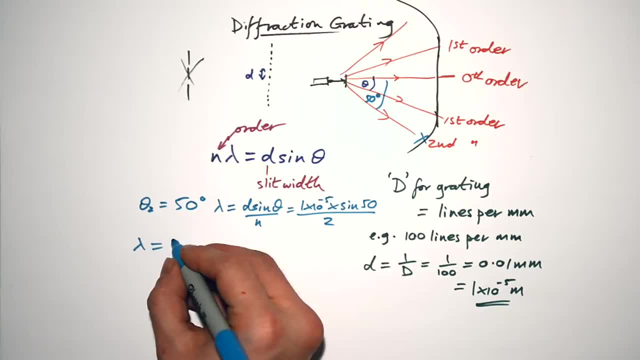 that's what I'm looking at. same up there. that gives you a wavelength of 3.83 times 10 to the minus 6 meters. now you could be instead be asked to find out the angle at which an order is at, so in that case you would have to do the inverse.